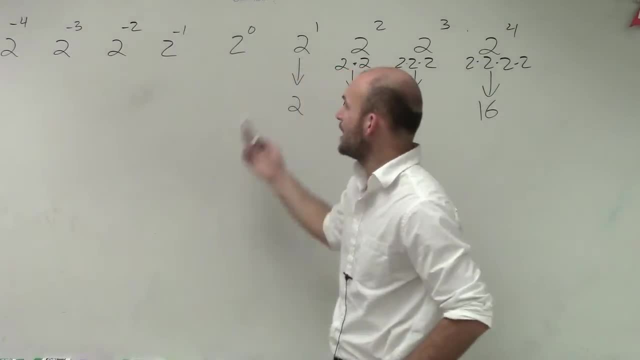 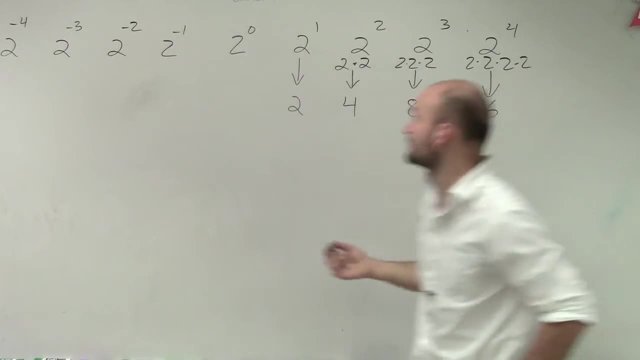 Now remember when we have the negative exponents. rather than multiplying by itself twice now, what essentially we're doing is we're dividing by 1 over 2.. 1 to the negative 2nd power means 1 divided by 2 to the 1st power. right, Remember, we put it in the denominator to make it positive. We showed y. when it's in the denominator, it's equal to that negative value. 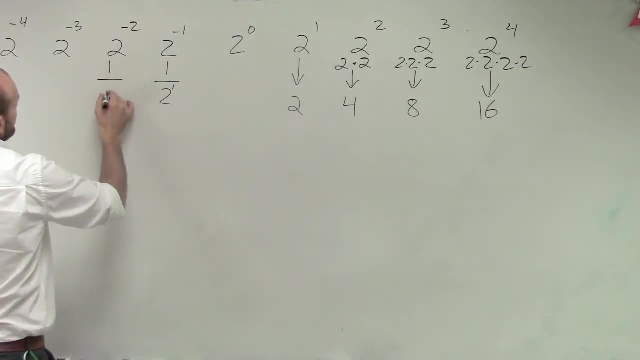 Then let's go and look at y to the negative 2nd, It's going to be y squared. So does everybody agree with me in my analysis right now? Okay, So this is really 1 over 2.. 1 over. 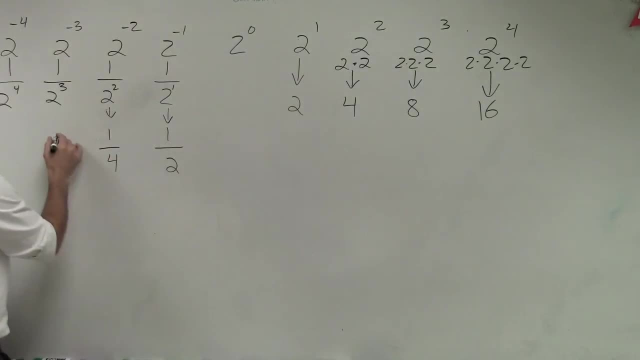 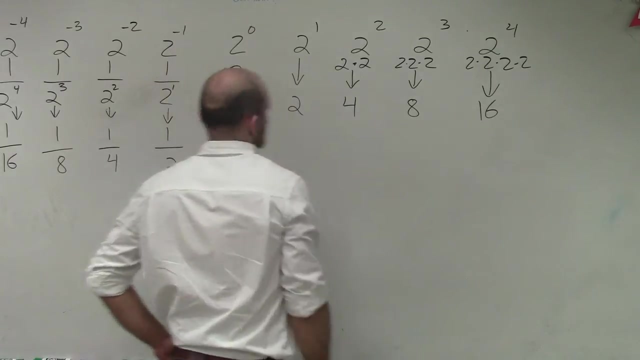 Teachers, pardon the interruption. I do have several bus changes this afternoon. Students who ride bus 274 will ride bus 637.. Students riding 202 will ride DS10.. Students riding 956 will ride DS12.. Students riding 202 will ride DS10.. 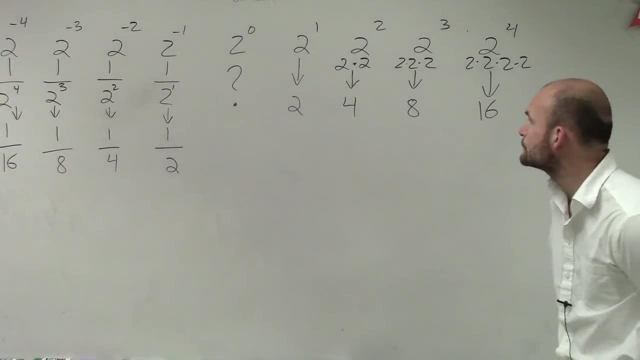 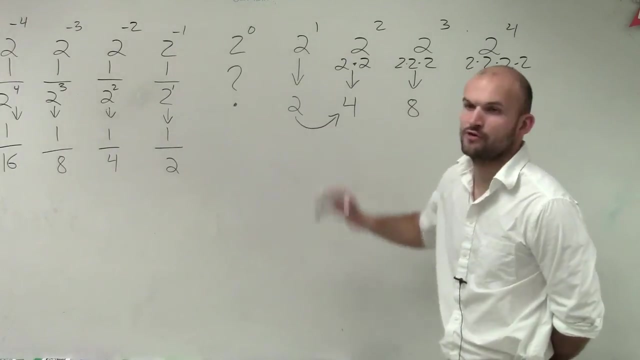 Students on 637 will ride DS4. Now Mallory, And students riding 274 will ride bus 637.. To go from here to here: what am I doing? What am I doing? To go from here to here. what am I doing? 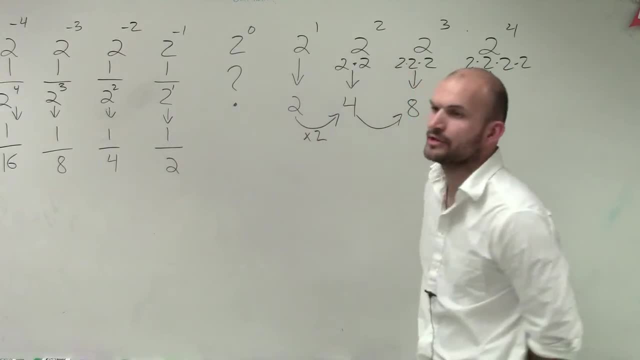 Multiply by 2.. Very good, To go from here. what am I doing? To go from here to here. what am I doing? Let's go back over here. To here to here. what am I multiplying by? You want to make sure of it. 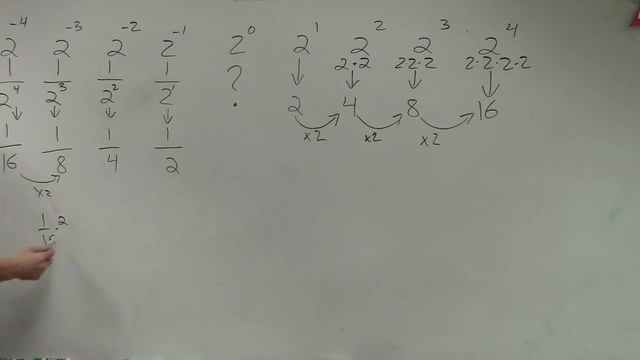 1 over 16 times 2 equals 2 over 16, which reduces down to 1 over 8.. Does everybody agree with me? This is the very, very important part that you're missing, Okay. So therefore, over here again, you're multiplying by 2.. 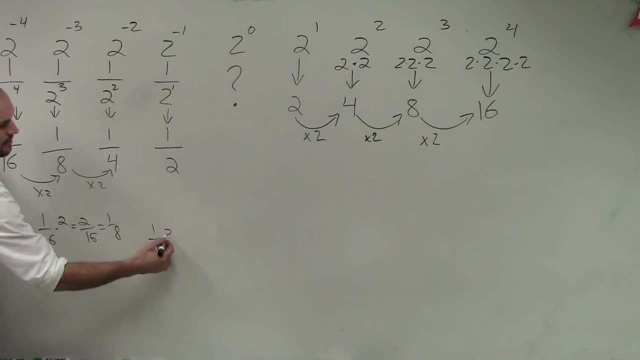 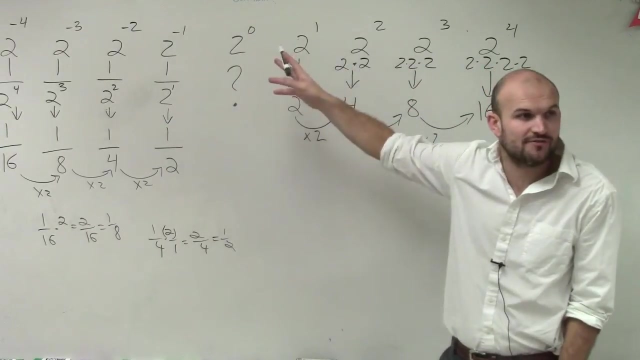 1 fourth times 2, is what? 2 over 4, which equals 1 half Chase. could you move please Now? so, ladies and gentlemen, if I'm looking for this next answer, right, If we're saying 2 to the negative second, negative first, then the next point up is 0, and then we go to the first. 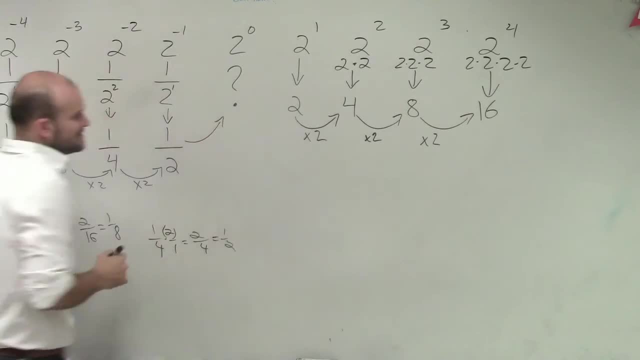 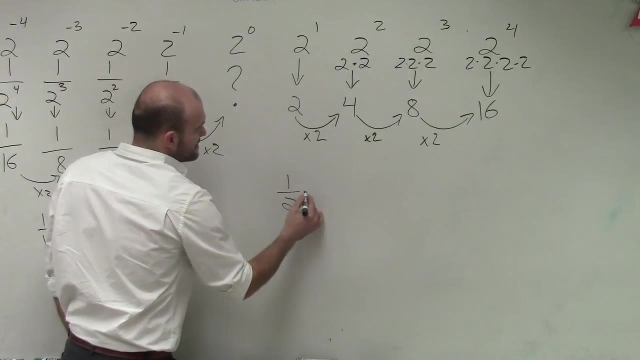 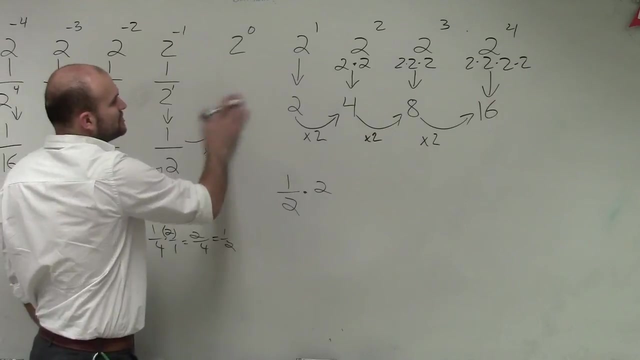 So what do you think I'm going to have to do to get to this next value, Multiply by 2.. So if I do 1 half times 2, what is that going to give me? 1.. So 2 to the 0 power equals 1.. 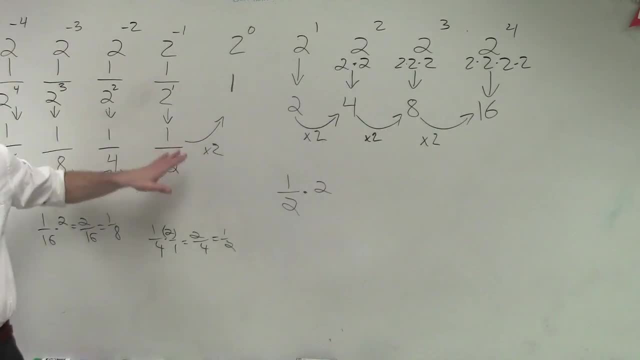 And guess what, ladies and gentlemen? I can replace all of these 2s with x's. I can replace all of these 2s with 8.. I can replace all of these 2s with x's. I can replace all of these 2s with 8.. 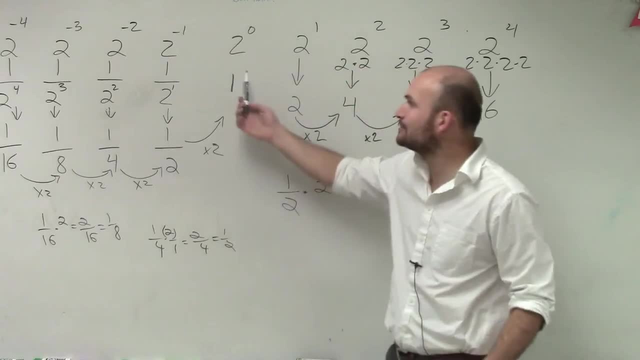 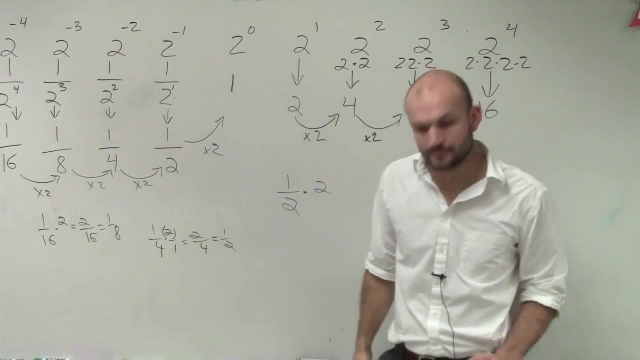 I can replace all of these 2s with a z, It doesn't matter. Anytime you take your base, raise it to the 0 power, you're going to get 1.. Okay Question. Well, when you said that anything raised to the 0 power was 1, I just believed you. I know. 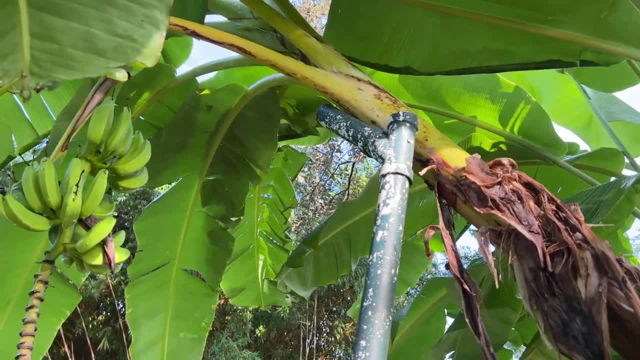 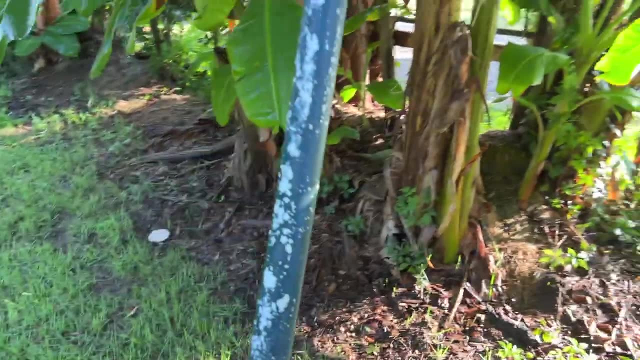 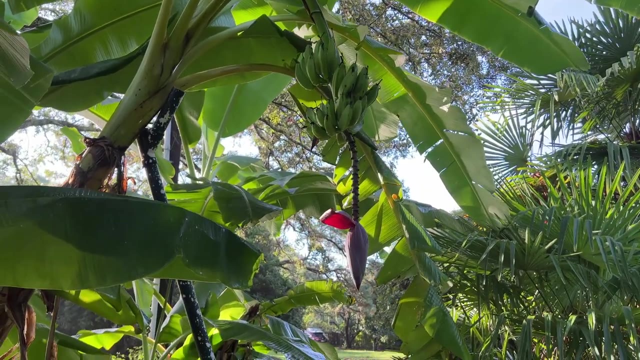 Hey, hey, this is Frank at Simply Bananas. Welcome back If you grow bananas in outside of Florida or some of the places like that. sometimes these bananas need a little bit of help as they grow along. This particular one has got a fairly heavy rack of bananas. 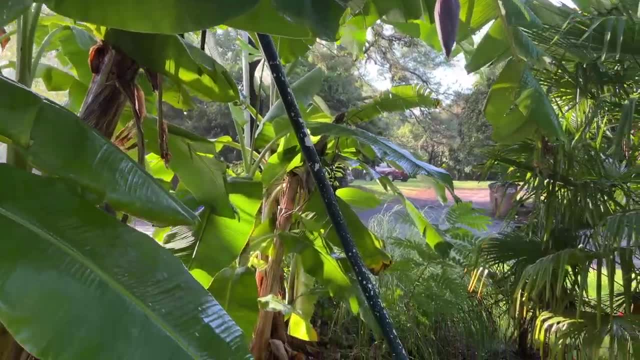 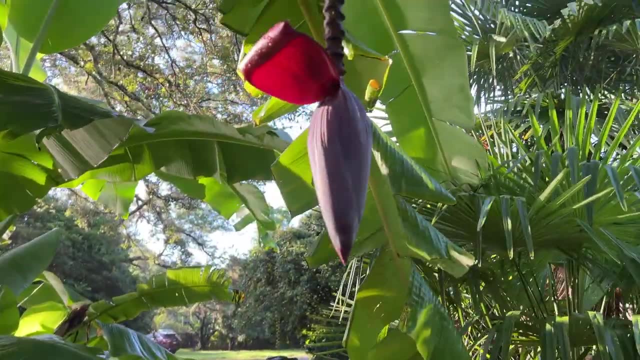 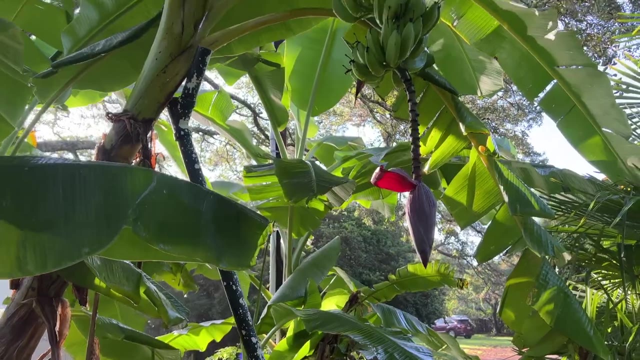 and the plant is leaning quite a bit. So you can see I've got a prop pole here. Now one of the things I'm going to do to help this banana plant survive is I'm actually going to remove this heavy flower. It can actually add almost a pound of weight to an already leaning banana plant, And